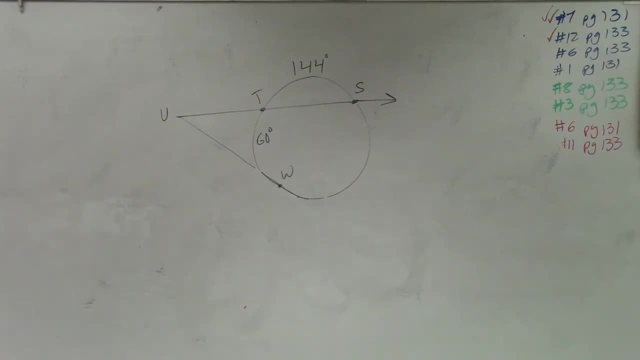 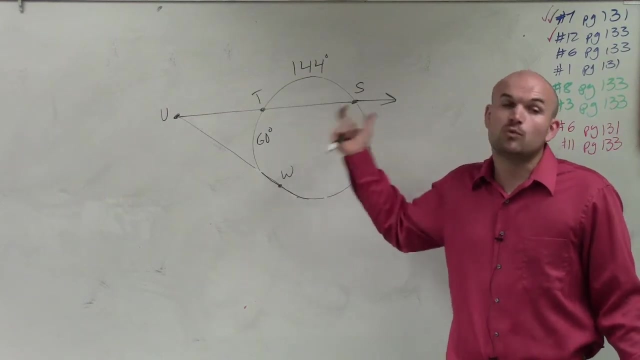 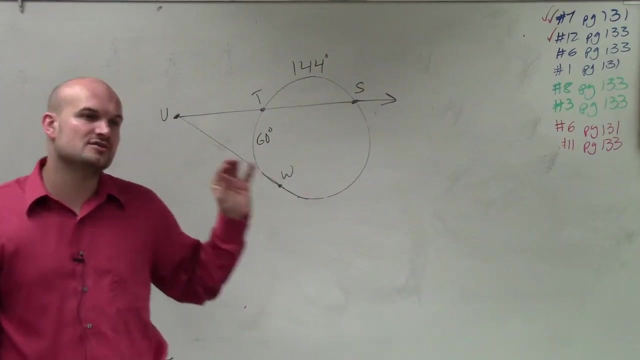 So in this example, ladies and gentlemen, when we were talking about points that were outside of the circle- So for page 133, there's a couple things we discussed. We discussed that when we have intersection, when we have angles of the intersection inside of a circle, that it's one half the sum of both arcs. We talked about when we had angles on the line, which is like a secant, which is one half of its arc measure. 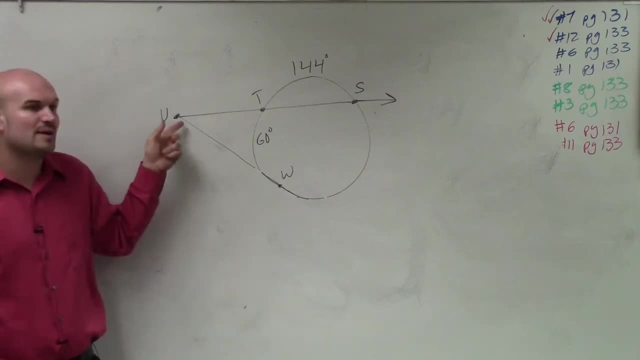 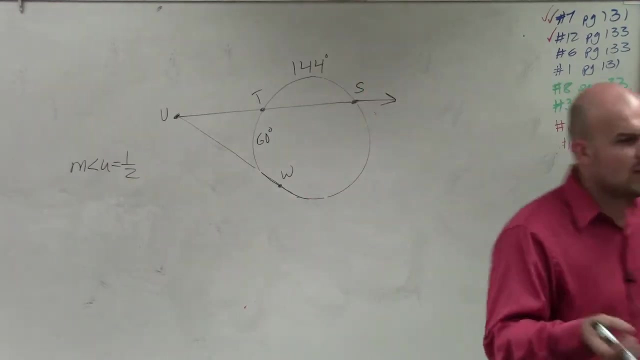 And then we talked about three different angles. when we had a point from outside of the circle, We talked about how do you find the measure of angle U if you had two lines that were secant, two lines that were tangent, or one secant and one tangent, which is, in this case, The formula for this, for the measure of angle U is equal to one half, If you guys can remember, whenever you have a point outside of a circle that is creating an angle and you need to find the measure of the angle when it's outside the circle, 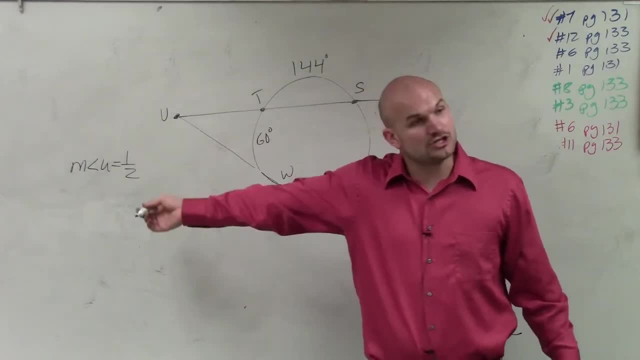 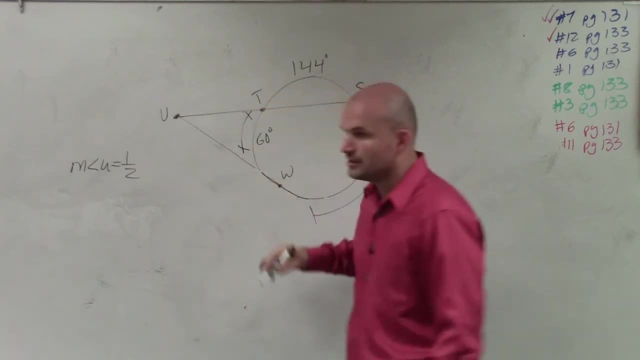 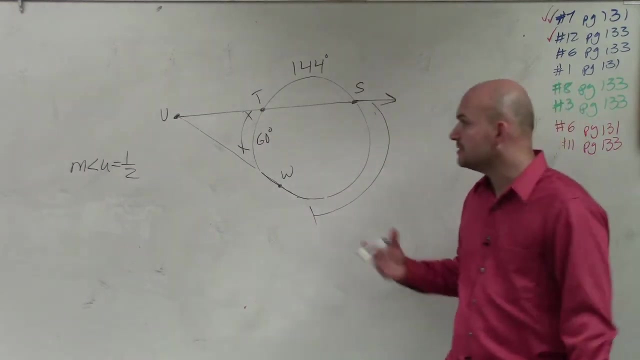 it's always one half of the large arc subtracted from the smaller arc, where here is my large arc and here is my smaller arc. When the angle was inside the circle, it was one half of the sum of the arc and its opposite arcs. So we need to be able to figure out what is SW. 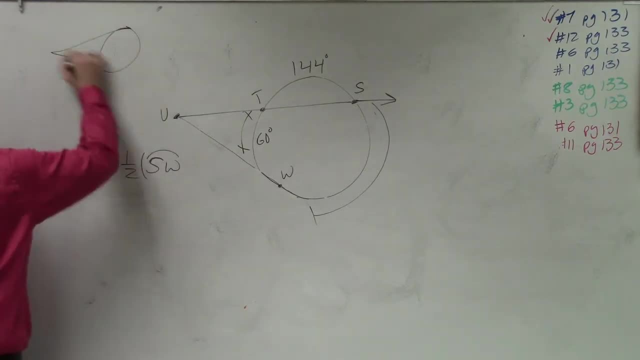 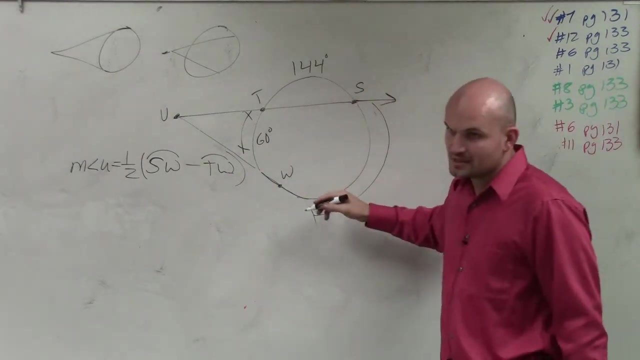 It's always for any point, It doesn't matter. We dealt with two tangents And two secants. It's always the large arc minus the small arc times one half. So it's SW subtracted from the arc TW. Now we know what TW is. That's 60 degrees, right, Good, That's easy. But we don't know what SW is. Now, fortunately for us, we know that all around the circle is 360, right, So I could say arc SW plus 144.. 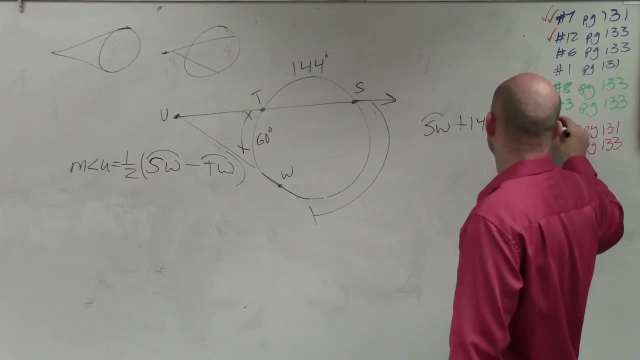 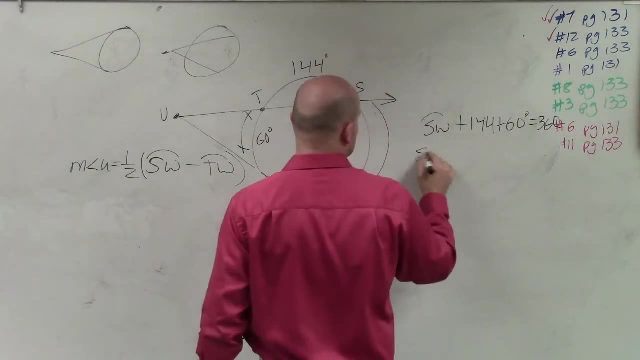 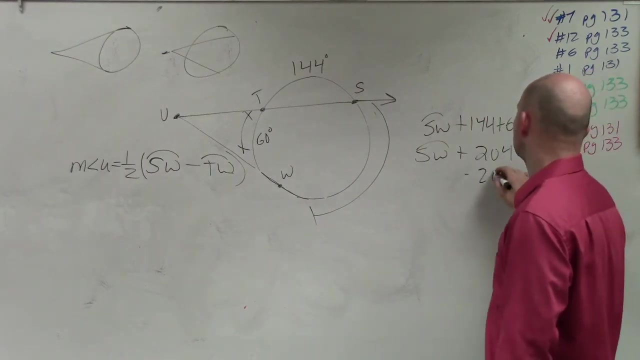 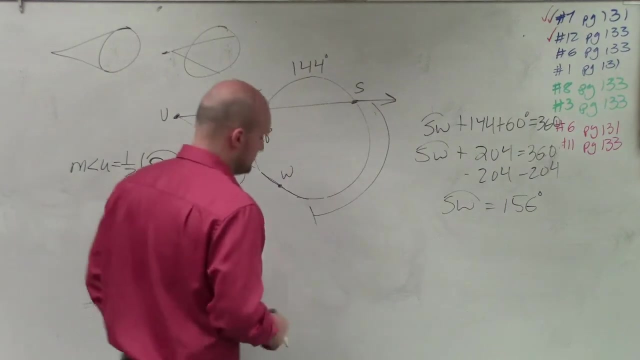 I need all of these arcs capitalized together, right? And when I get all of these arcs, how many degrees? Yes, I'm stopping you, I'm trying to write this down. So, according to the proposal table, if X, identical W plus 60 degrees equals 36 xu, right?